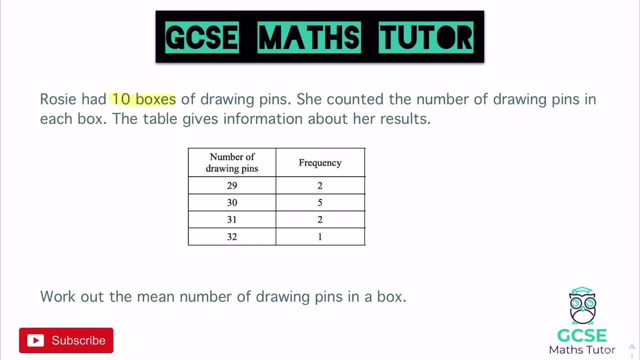 okay, but once we start getting to tables, where there's 80, 100 things in the table, we won't want to do it in this particular way, but just so you have an understanding of how and why we do the process we do, we'll have a look at this first one. So we've got two boxes of drawing pins that have 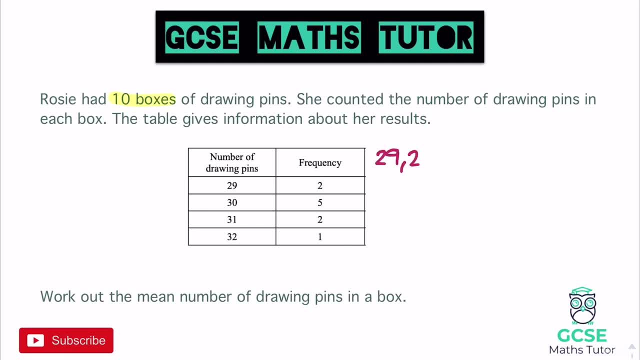 29 in, so we'd have two 29s, so 29 and 29.. Then we've got five with 30 in, so 30, 30, 30. You can already see it's actually already a bit annoying having to write these all out: 30 and 30, there. 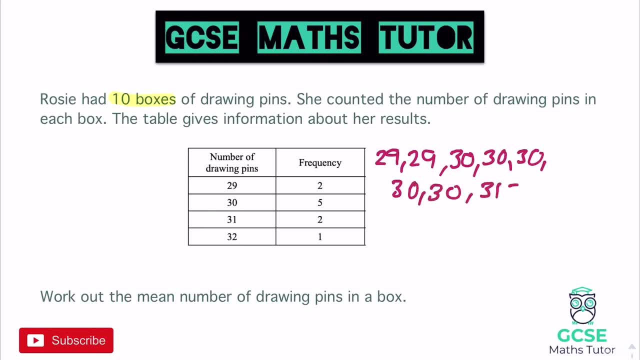 we go, We've got two with 31 and another 31 and we've got one with 32 in. So I could just give you this list here and say: work out the mean, and what you'd do is you just add them all up and we. 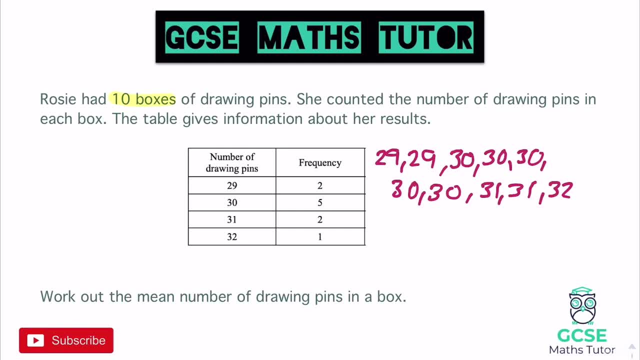 would divide by 10.. So with this particular table we could actually just take that approach. it'd be nice and easy to do that. So we've got two boxes of drawing pins that have 29 in. so we'd have two boxes of drawing pins that have 31 in and we would divide by 10.. So we've got two boxes of 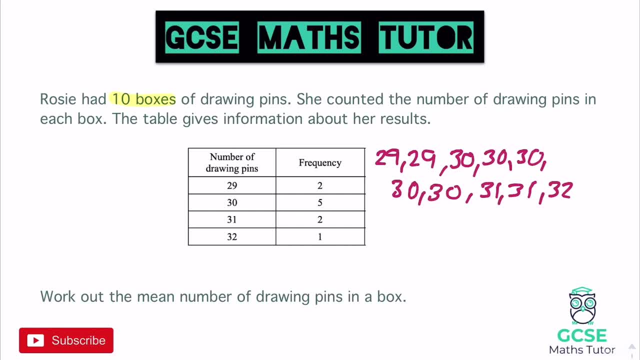 drawing pins that have 31 in, and we'd have two boxes of drawing pins that have 31 in and we'd obviously, as I said, as they get a bit trickier, we're not really going to want to take that approach, But essentially we're going to have a look at what the totals of all the numbers are. 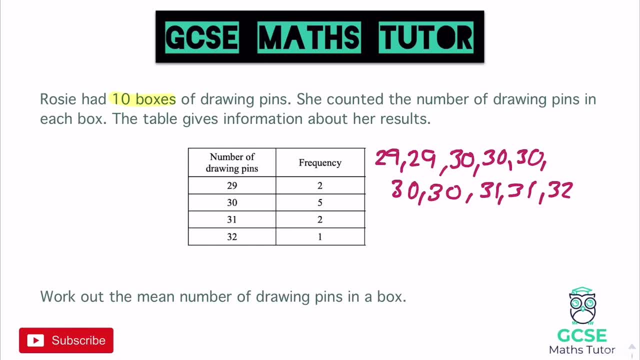 and what we're going to do, obviously, because they're categorised. what we're going to have a look at is we're going to look at the total of these 29s. to start with. Now, there's two of them, so two 29s. we could add those together and we get a nice total there, and that is 58, that total. 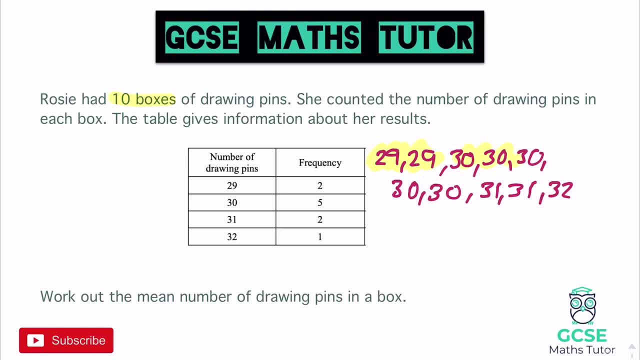 Then we would have a look at the 30s and we'll add all of those up. We've got 30, 60, 90, plus of the two 120, 150.. So the total of those is 150.. The total of the 31s is 62. And the total 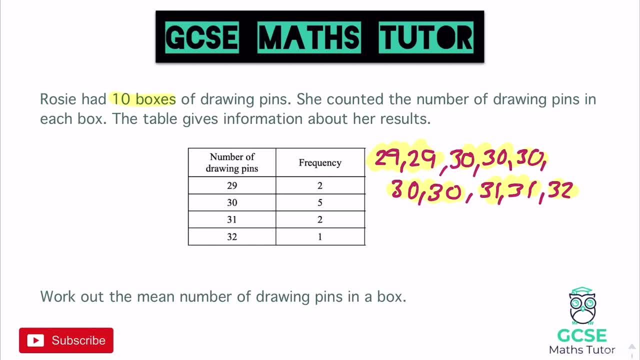 of that 132, there is 32.. And then we can add them all together as groups. What we're going to do is we're going to take that away from the list and have a look at it from the table, So we'll get. 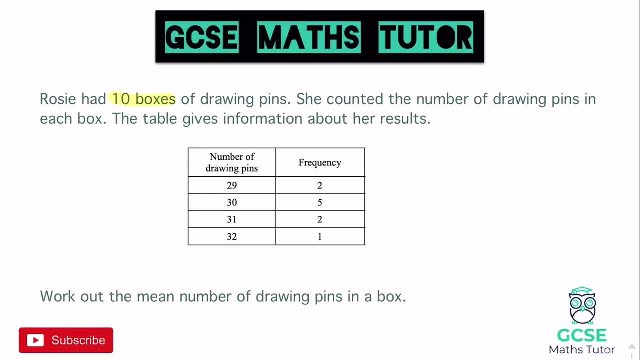 rid of all of that, And we'll do it from the table here. So we've got two 29s. Now all we have to do is times the 29 by two And that gives us their total there. So two lots of 29,. we've already said 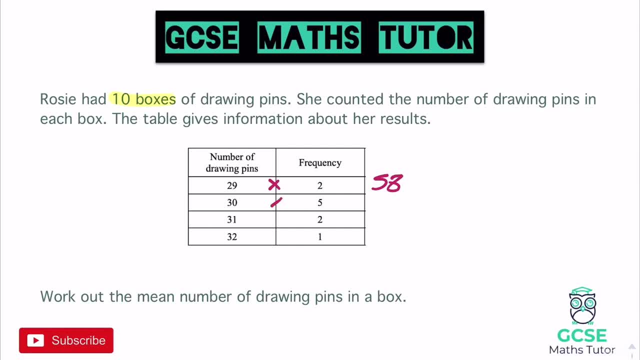 is 58. Then we've got five lots of the 30s, And that was 150. And we've got two lots of the 31.. That's 62. And one lot of the 32. And that gives us 32 as the total. there Now, throughout these, 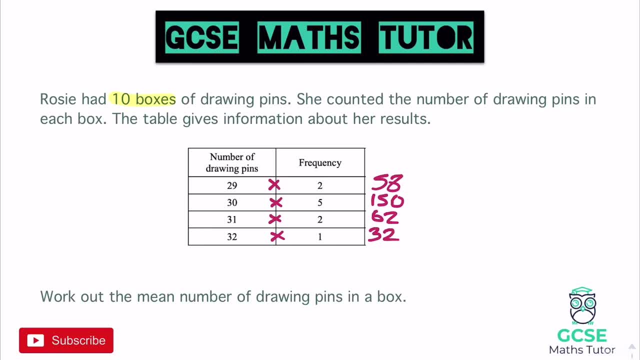 questions. they could be calculator, They could be non-calculator. I am just going to use a calculator, Although I've got to be honest. I think this question is a good non-calculator question. But as long as you know the process, obviously, if it was a calculator question it would be quite. 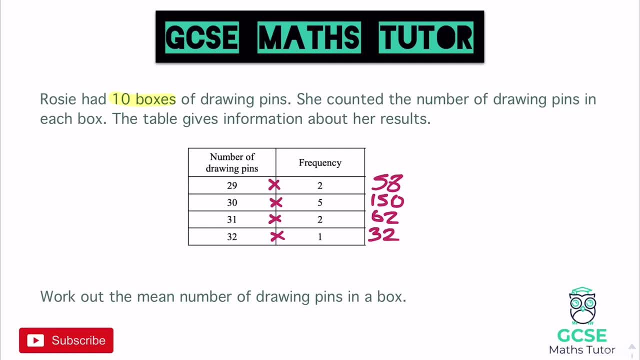 nasty One that you wouldn't be expected to do without a calculator, but they could be non-calculator as well, And here's an example of one, I think, where this could be non-calculator. So let's have a look. Now we've got all these totals for each row. We can actually just add those all together, So 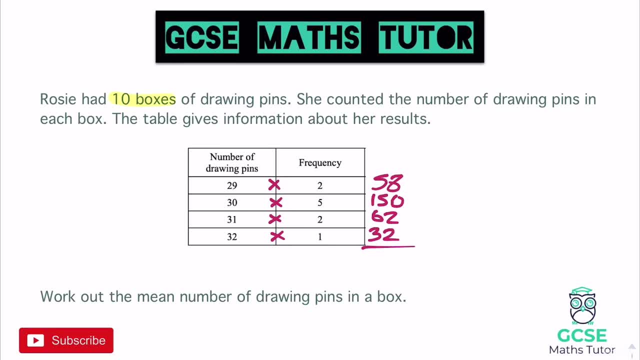 58 plus 150 plus 62 plus 32, gives us the overall total there of 302 for the total number of drawing pins in all these boxes. Now we already know we're going to divide by 10,, as it says in the question up there, that there's 10 boxes. But if we're going to divide by 10, we're going to 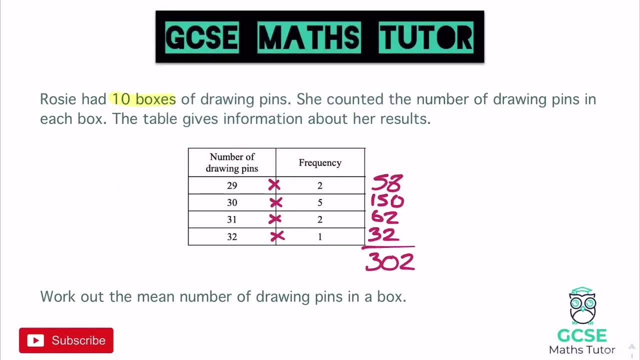 divide by 10.. So if we didn't actually have that piece of information, we could find that, because we've got the total frequency just here And if we do 2 plus 5 plus 2 plus 1, we get a total of 10. 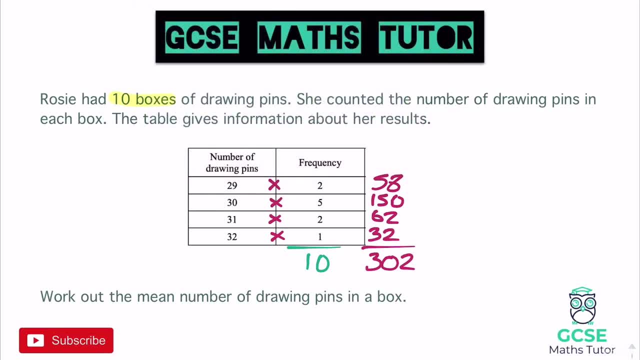 boxes. So all we need to do to finish this question off, to get our value of the mean, is we're going to do 302, the total of all the drawing pins, and divide it by the 10 boxes, As you can see that. 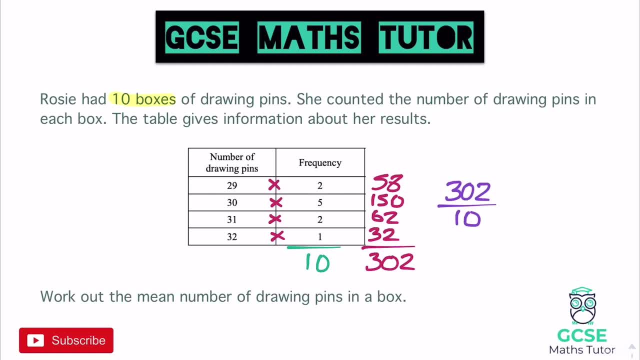 would obviously be why this might be a non-calculator question, because dividing by 10 is nice and easy. We just hop the decimal in and we get the answer: 30.2 for our mean. So in terms of a process there, look we times across, we get all the totals for each category. We add them all up and divide by how many things there are- And in this case the things is the 10 boxes- And we get that just by adding up the frequency column down here. So there we go: get the total divide by the total frequency and you have got your mean. Now you're going to have a go at a couple of questions. So here are some for you to have a go at. 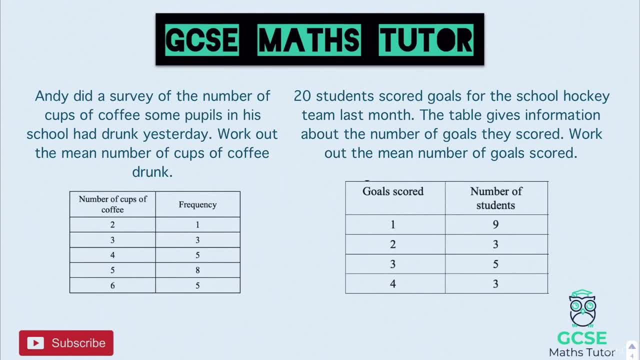 Okay, so there's two different questions here with two different contexts. So have a read of the question, have a go at working out the mean for each one and we'll go over the answer in a sec. So pause the video there and we'll go over the answers. 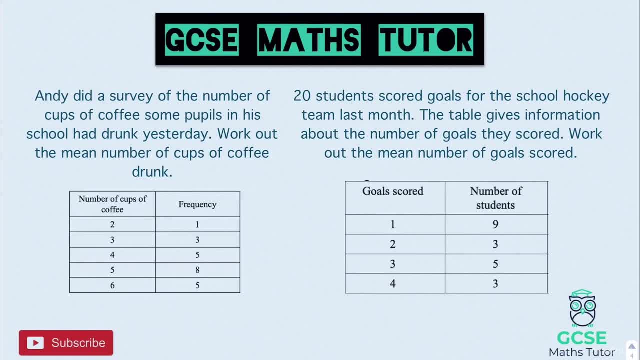 Okay, so this first one we've got. Andy did a survey of the number of cups of coffee some pupils in his school drunk yesterday. work out the mean number of cups of coffee drunk, So we're going to times them all across to start with and we'll get all the totals for each of our rows. So 2 times 1 is 2,, 3 times 3 is 9,, 4 times 5 is 20,, 5 times 8 is 40, and 6 times 5 there is 30. And if we add those all up, 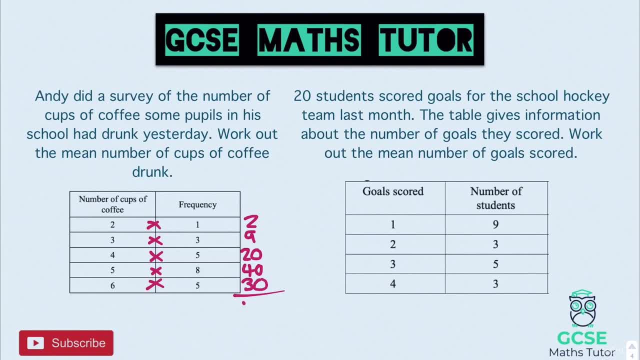 40 plus 30 gives us a total of 101.. There we go, and if we add up our total frequency- as it doesn't tell us in the question how many people there are- 1 plus 3 plus 5 plus 8 plus 5 gives us a total of. 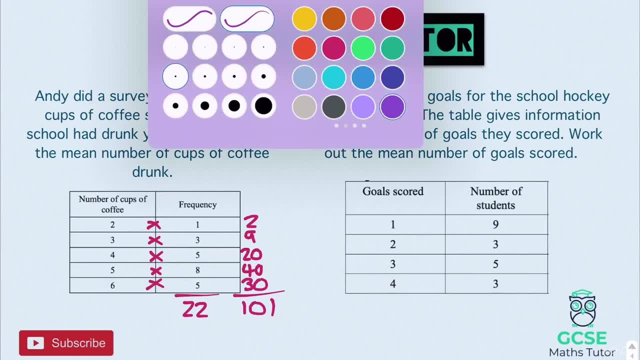 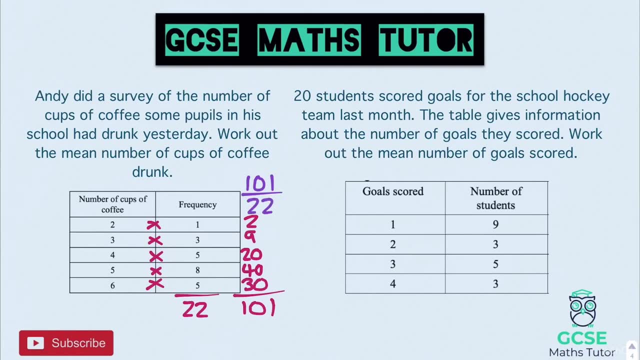 22 people. There we go. so this is definitely a non-calculator question. we're not going to do 101 divided by 22, so let's just do that on the calculator, 101 divided by 22, and let's see what we get: 101 divided by 22 and we get the answer of 4.590.. Let's see if I can squeeze that in. 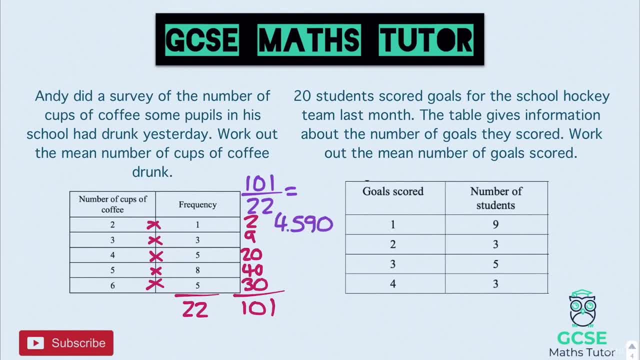 4.590, and there's a recurring decimal of the 9 and the 0, so there's a recurring pattern of 90s there. and that would be my answer: 4.590 and there we go. Okay, obviously it doesn't say to round it. 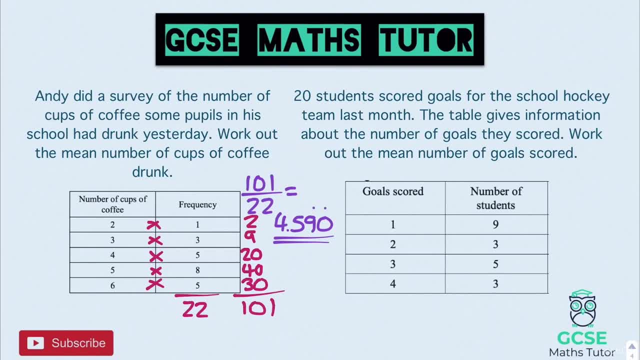 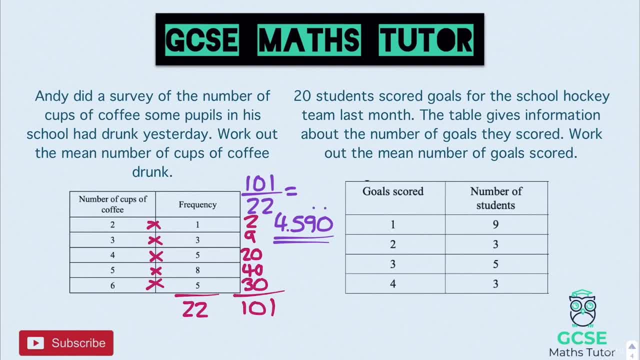 about the logic. it does say: work out the mean, which is the average, and four and a half makes sense. Okay, look at the number of cups of coffee drunk. they ranged from two down to six and it's somewhere in between there: 4.59. that makes sense, as it looks like between four and five is the most. 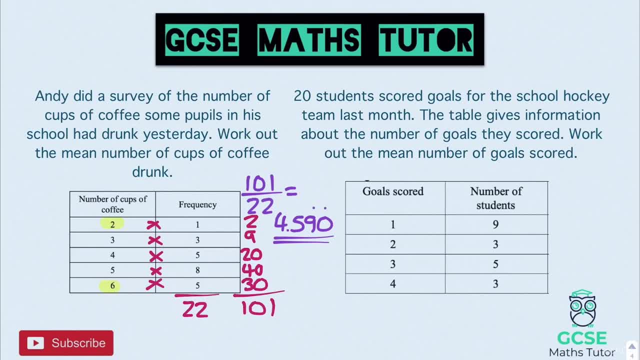 common amount of cups of coffee drunk there as well. so that makes sense. On to our next one. let's times these across. so it's about goals scored in 20 matches. 20 students actually scored goals for the hockey team and it says: this table gives you the number of cups of coffee drunk. 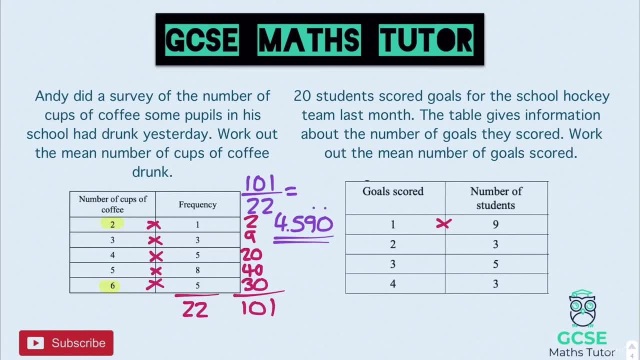 they scored. so one times nine gives us nine. two times three gives us a total of six. three lots of five is 15, and four lots of three is 12, and if we add those all together, 12 plus 15 plus 6 plus 9. 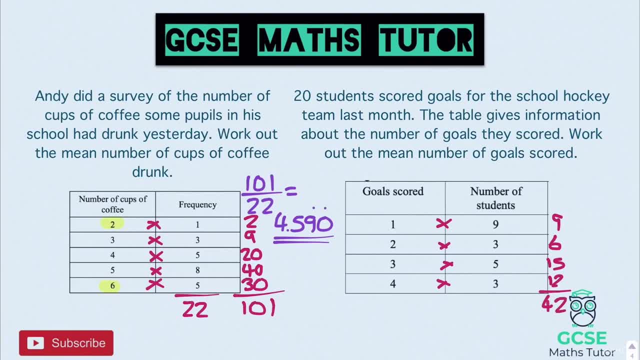 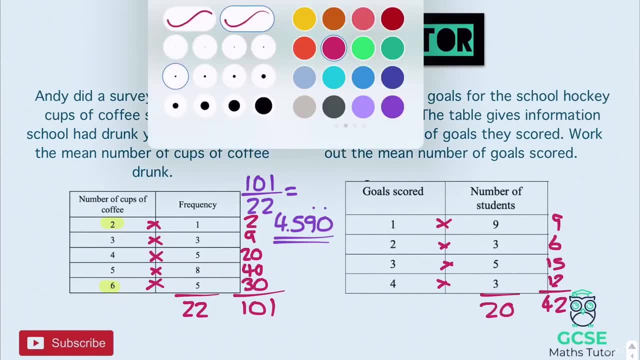 gives us a total of 42.. There we go, and we already know there's a 20 total here, so we can just add those up. but just double check they do add up to 20 and then we go and we can finish this off. we've. 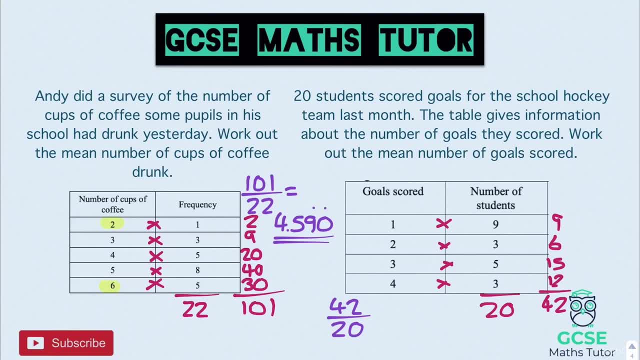 got 20 people to divide by, and 42 divided by 20 is 2.1. and again, looking at the context of the question, 2.1 goals makes sense. there we go and there is our final answer and our mean for that second question. Now let's have a look at some group frequency. Okay, so that group word I've 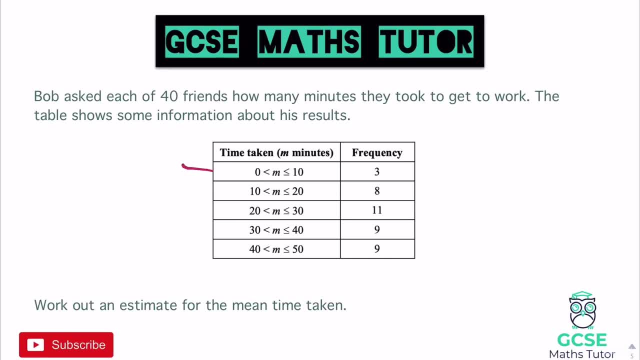 mentioned. grouped frequency refers to these categories here. so this question is about 40 friends and how long they took to get to work. So we've got a category there and that means from 0 to 10 minutes, including the 10. okay, obviously not including the 0 there, because no one's going to take 0 minutes. so it's anywhere between 0 and. 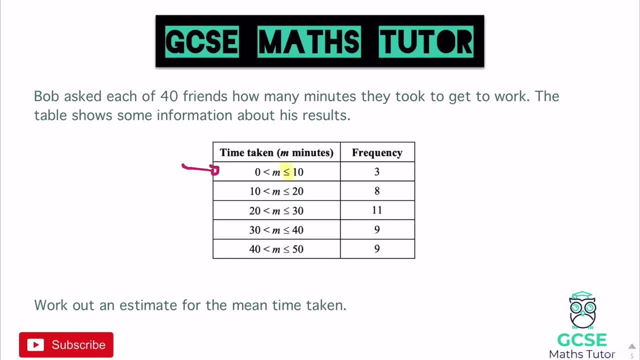 10 and obviously that little symbol there, the equal to symbol, tells us it can actually be equal to the 10.. The one below then look, starts on 10, but obviously it's got that not equal to 10 there. so obviously anyone that's on 10 minutes exactly would go into the category above where it. 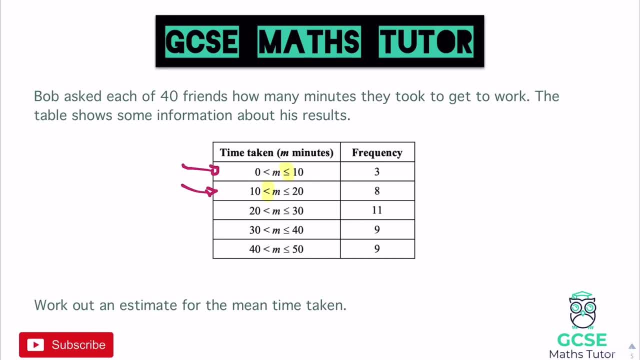 can be equal to 10.. So that can't be equal to 10, but it's between 10 and 20.. And again it can be equal to 20, and that sort of pattern there just follows all the way down the table. the next one: 20 to 30, not including 20, but does include the 30. Okay, so that's what those 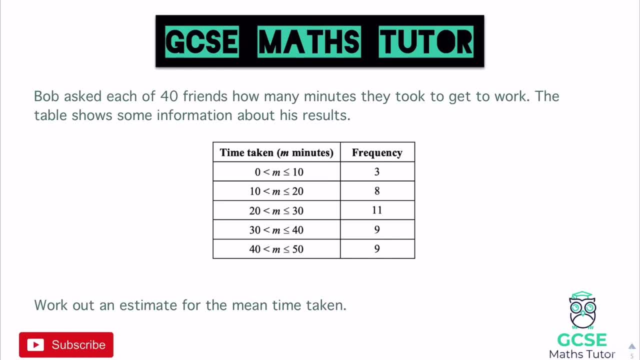 little inequalities are those little groups and it's called group frequency. but these little things here are also called classes or it's called a class. okay, and think about that word class. if you're in a class at school, that refers to the group that you are in. so another word for 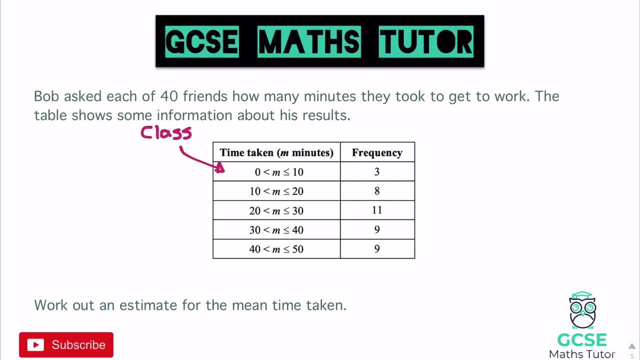 group is a class and we're going to refer back to that word later on in the video. So this sort of question here. basically, we don't know how many of these three people. well, where they're actually at in terms of their minutes, they could be one minute, two minute, three. 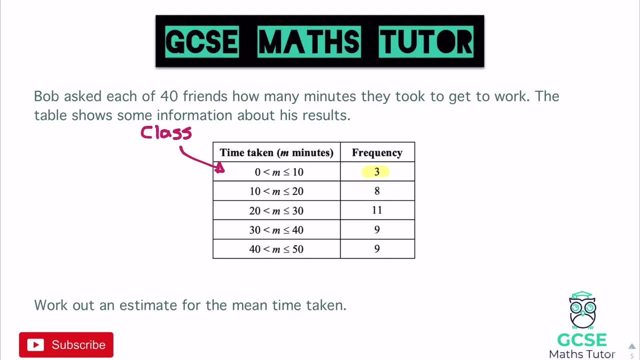 minute, any sort of subcategory of that, as it could be four minutes 50 seconds. it could be anything within 0 to 10 minutes, so essentially we don't actually know the times within the group. although we know that there are three people within that group, we don't know their exact times. 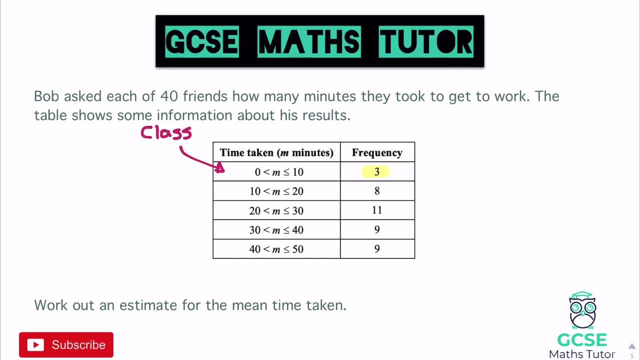 So the question down here? look, in this final line it says it's something different. in the words it says: work out an estimate for the mean time taken. And we're working at an estimate because we obviously don't actually know their exact times. if we did know their exact times we could calculate or work out the mean, but for this particular 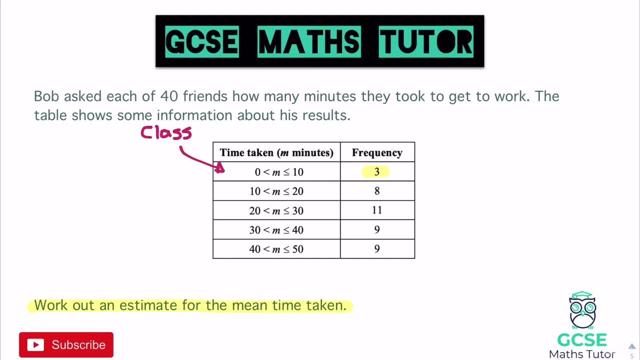 question. we're going to estimate the mean. So, in terms of actually making an estimate, what we're going to do is we're going to make a guess for these people's times, obviously an educated guess- between 0 and 10. the midpoint, or in the middle of that, is 5.. So we're going to use 5 instead of any. 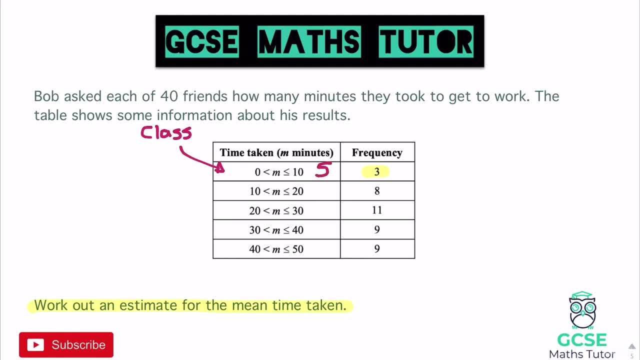 of these random numbers in between 0 and 10.. So say, okay, 10, 5's in the middle, so we use that. in the middle of that is 15, so we use 15 for that category. 25 between 20 and 30. 35 between 30 and 40. 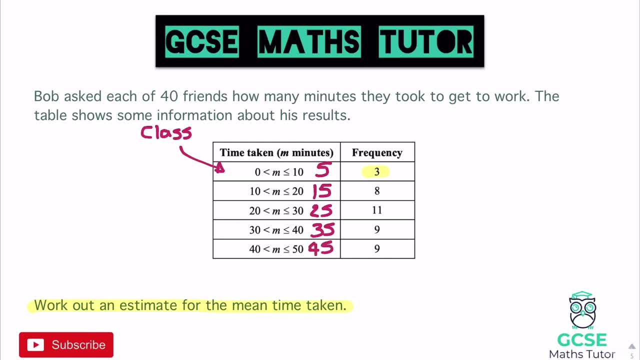 and 45. between 40 and 50. Now I've assumed there that you can spot those in your head. if you can't, let's have a look at this category, for example: 20 to 30. you could just add together 20 and 30. 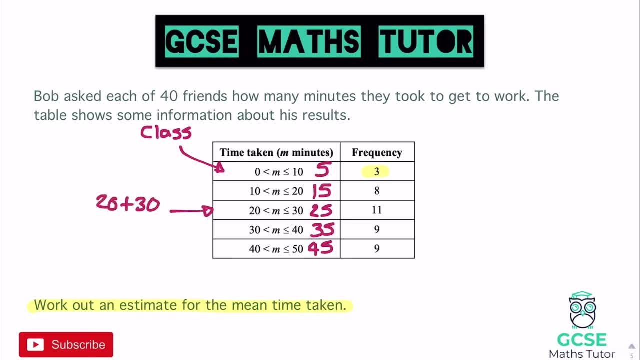 you could do 20 plus 30 and then half your answer and again, 20 plus 30 is 50, half it is 25 and it gives you that midpoint. So if they are a little bit more complicated and you're not sure what, you can't spot them in your head. there's a little trick for you: just to find the midpoint, okay, and 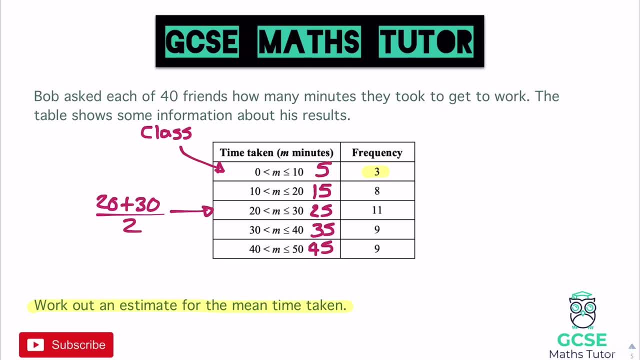 you can do always use that to find the midpoint of two numbers as well. Now we just follow the same process. so now I've got my estimated midpoints, or my estimated times in the context of this question, I'm just going to times them all across, like we did before, and the rest of the process is. 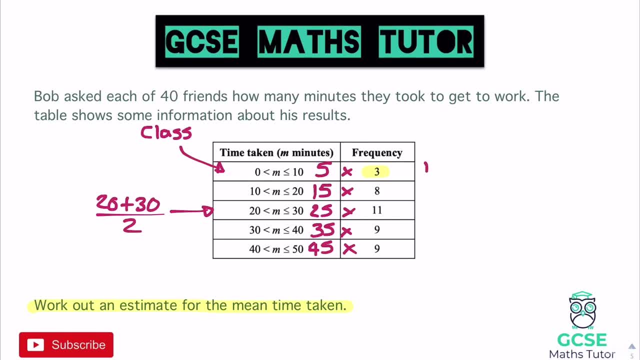 basically exactly the same. So 5 times 3 is 15,, 8 times 15 is 120,, 25 times 11- and I am doing these on the calculator- is 25.. So I've got my estimated times in the context of this question and I'm 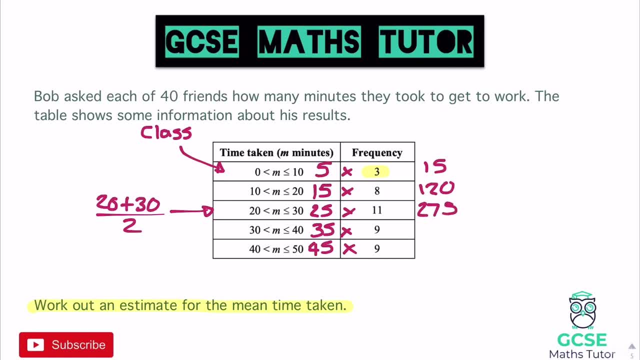 just going to add those all together and get our overall total. So add 405, 315 plus 275 plus 120, plus that 15 sitting on the top, and that gives us a total of 1130, and that is our overall total there. 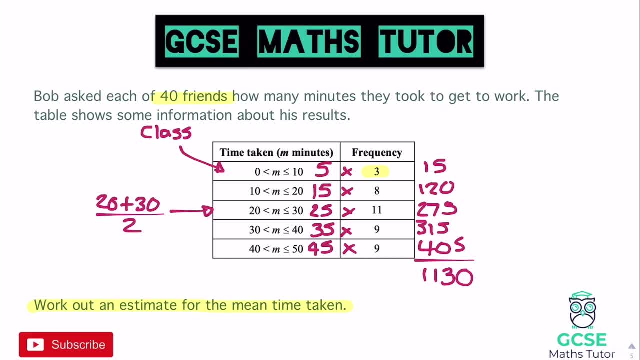 Now again, this question does say there's 40 friends, but again, just double check and add that all together down the bottom here and the total frequency there does add up to 40. so it's all okay. and again, we just finish this off, finishing off the working out, just like we did before. we've got. 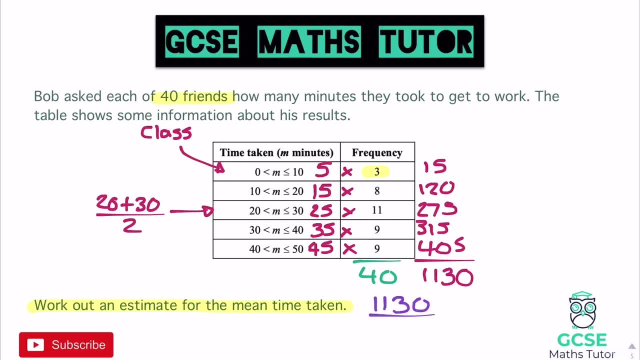 our big total, 1130, and we're going to divide that by the 40 people and see what we get for our estimated mean. So dividing that by 40 on the calculator gives us a final value of 28.25.. Obviously, the context of this question is about minutes, so it's. 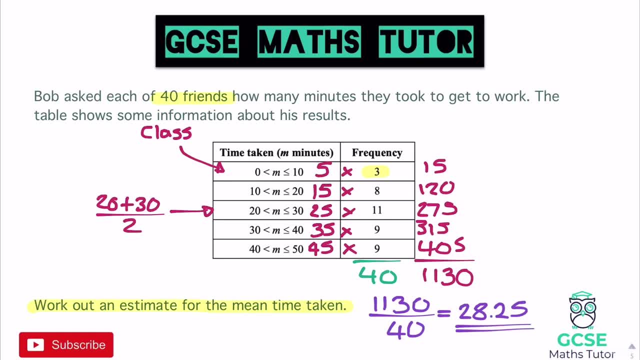 28.25 minutes, but that is our final answer there. and again, just looking back at the table, 28.25 makes sense. It's somewhere in this middle category here which is also the most popular. okay, obviously there's 11 there, so that would make sense that the average or the mean would. 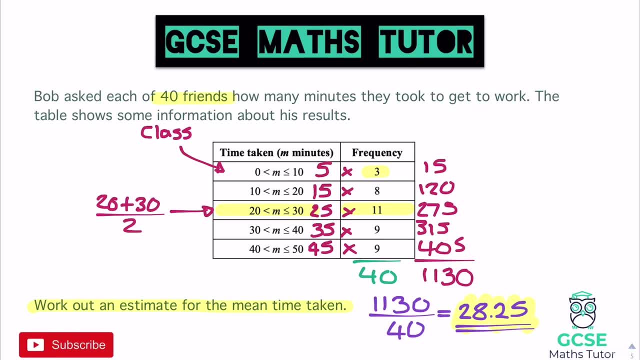 be within that category as well. So there we go. that's how to get an estimated mean from what we call a grouped frequency table. Don't be put off by that word grouped frequency. it just refers to these tables here where we have a class interval there and not actually a group. 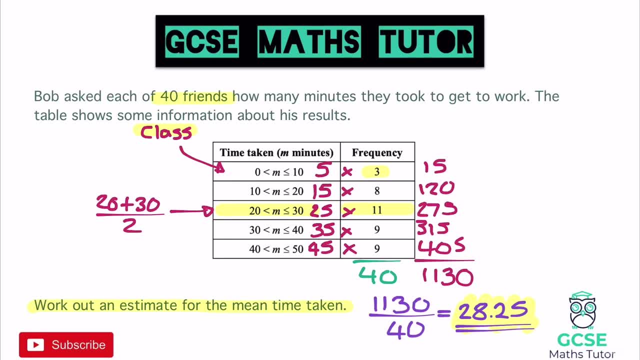 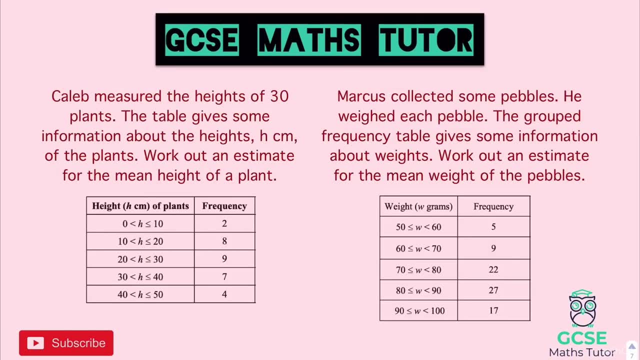 It's basically just a number within that. Okay, so that is how you work out an estimated mean, and here's a couple for you to have a go at. Okay, so there's two questions there, so have a go. pause the video and we'll go over the answer in a sec. 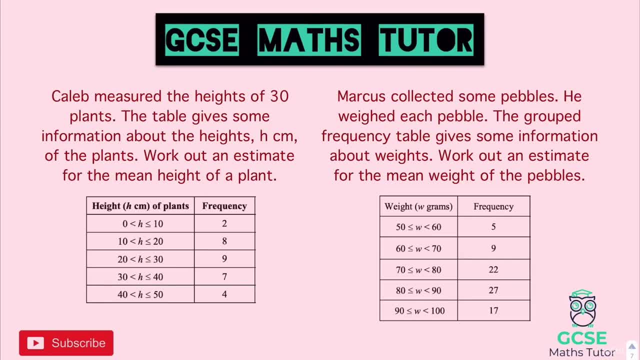 Okay, so this first one. first of all, the midpoints. we've got 5,, 15,, 25,, 35 and 45, and we're going to times all of those by the frequency. There we go Right. so 5 times 2 is 10,. 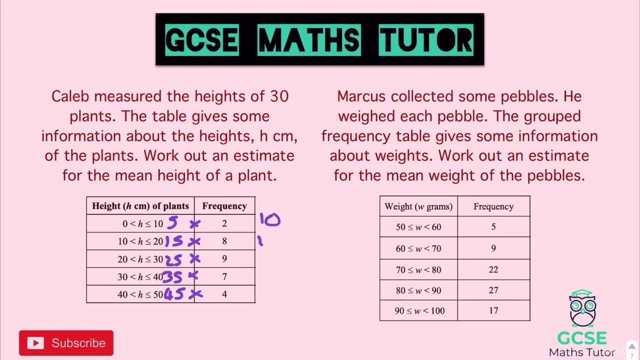 8 times 15 is 120, 25 times 9 is 225, 7 times 35 is 245 and 4 times 45 is 180.. There we go, and if we add those all together, let's see what we get: 180 plus 245 plus 225 plus 120. 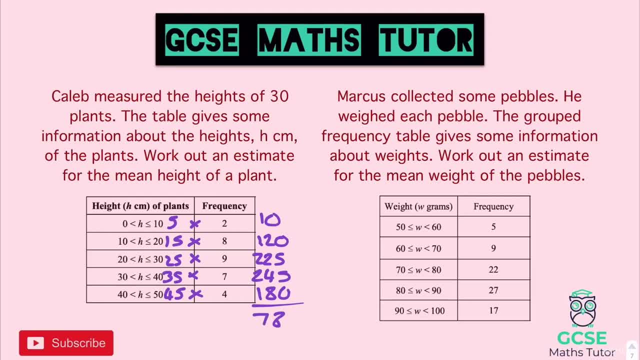 and add the 10 and that gives us an overall total of 780.. Now again, it does say in the question that there's 30 plants in this particular question. so if we add those all together we've got 30 and we just need to get our mean now, our estimated mean. so we're going to do 780, our 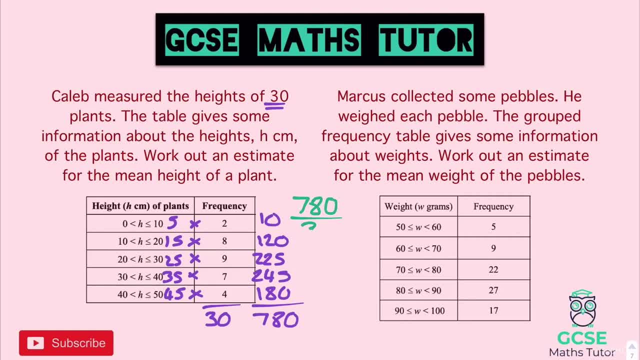 overall total. we're going to divide that by the 30 plants and let's see what we get: 780 divided by 30 gives us a total or an estimated mean here sorry- of 26.. There we go. and then again, thinking about the logic, look that sits within this category here, which again is the most popular. So again, 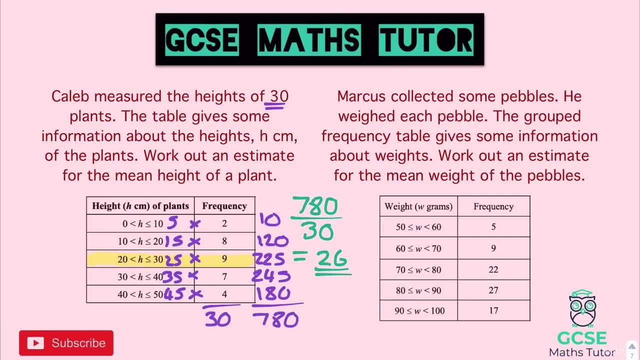 that makes sense and it's somewhere in the middle there, so that would make sense there for our final answer. so 26 is our mean. Moving on to our next one, we've got 55 in the middle of 50 and 60.. I'm 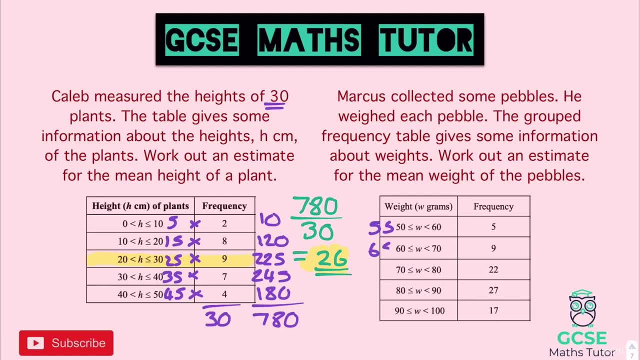 going to put these to the left. this time 55, we've got 65,, 75,, 8. that does not say 75, 75,, 85 and 95 in the middle of that last category. Again, times these all along we're going to get. 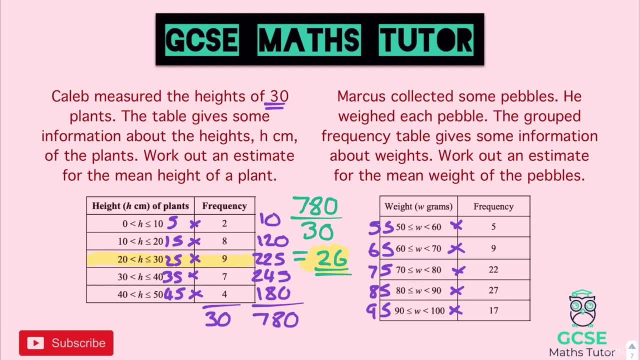 some quite big numbers for this one. let's have a look. So we have 5 times 55, and that's 275.. There we go. we've got 9 times 65, which is 585.. There we go: 22 times 75. 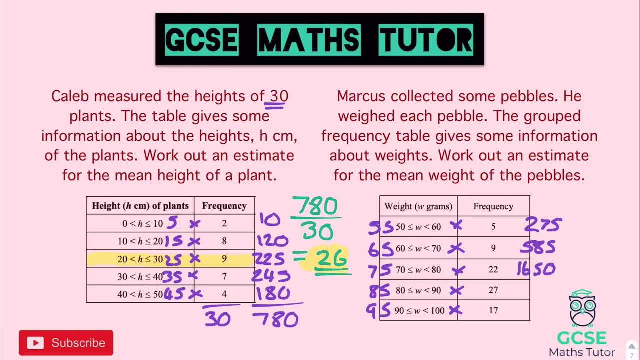 which is 1650.. 27 times 85, which is 2295.. There we go. and 17 times 95, which gives us 615. and you can see from this example here, this particular question, why we definitely wouldn't want to use a list. okay, because obviously we've got quite a lot going on in here. 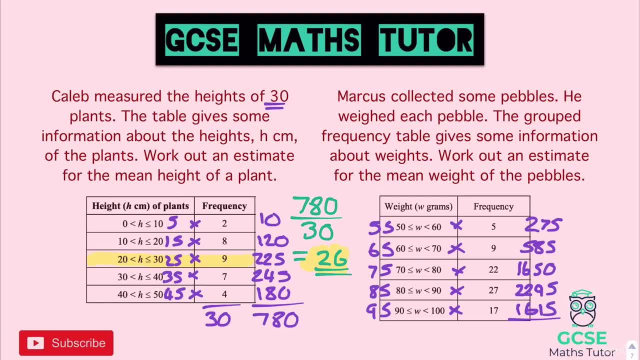 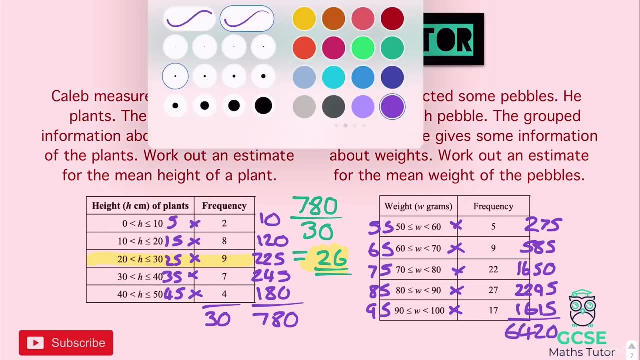 Now, if we add those all together- 1615, add the 2295, add the 1650, add the 585 and finally add the 275, we get a total of 6420.. Now again, we need our actual overall total amount of plants here. so if 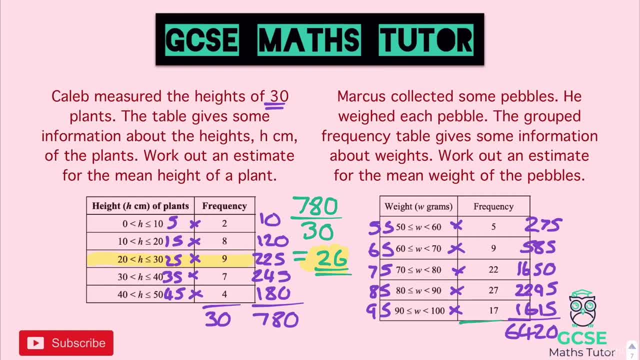 we look at our frequency column, 17 plus 27 plus 22 plus 9 plus 5 gives us a total of 80. There we are, we have a total of 80. So, working out our mean for this, we've got our overall total. 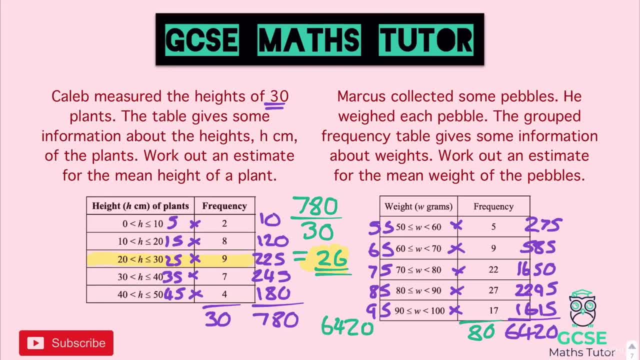 which is 6420, and we're going to divide that by our 80 there and if we work that out, 6420 divided by 80, we get our estimated mean, which is 80.25.. There we go And again thinking about the context of the question, 80.25 is in this category here, which? 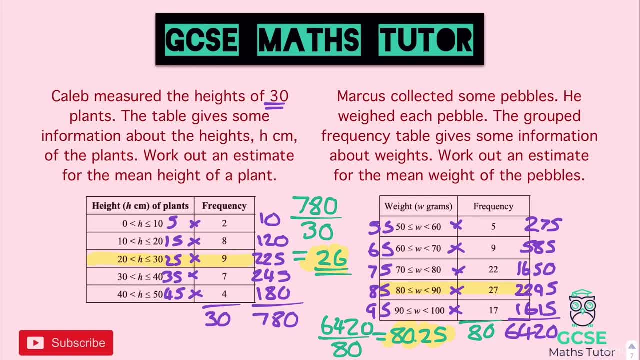 again just happens to be the most popular. So there we go. that's how you get your estimated mean from a table. So what we're going to have a look at now is some of the other averages. Primarily, we're going to look at mode and median, but we're also going to have a little quick. 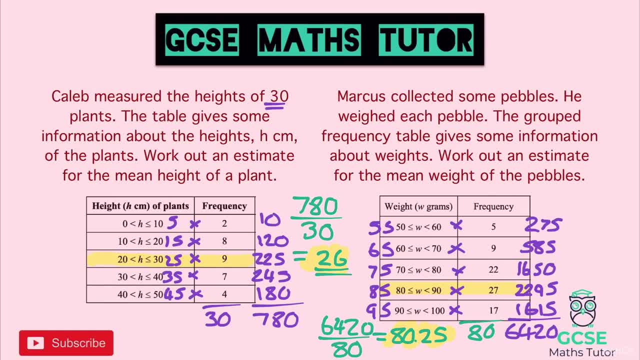 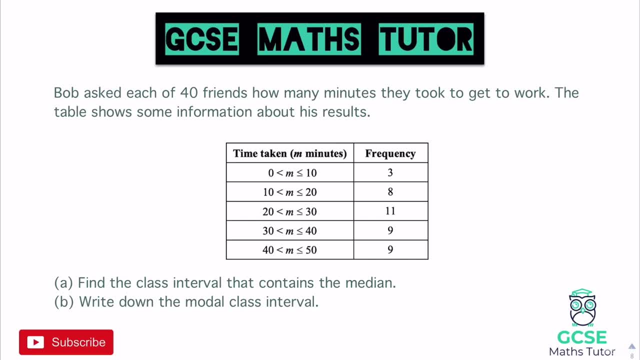 discussion about the range as well, and the range is quite nice and easy. Okay, let's have a look then. Okay, so we look. just looked at this question previously. Okay, it was about Bob asked each of 40 friends how many minutes they took to go to school. 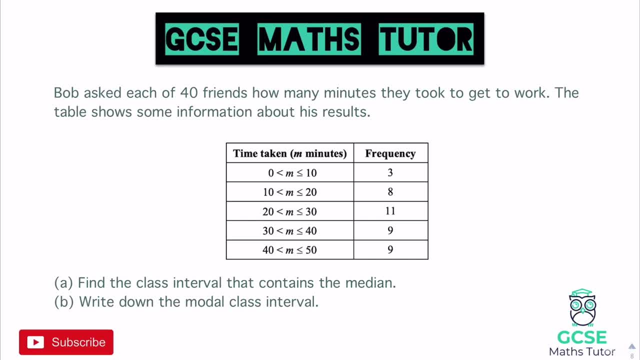 Okay, it was about Bob asked each of 40 friends how many minutes they took to go to school. Okay, it was about Bob asked each of 40 friends how many minutes they took to go to work. The table shows some information about his results. 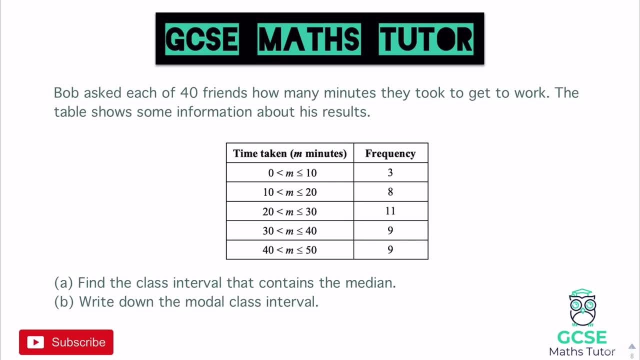 We're obviously we're going to look at these in separate parts, so we're going to start by finding the class interval that contains the median. Now again that language. there, class interval just means the group. okay, this one here that contains the median, the group, the interval. 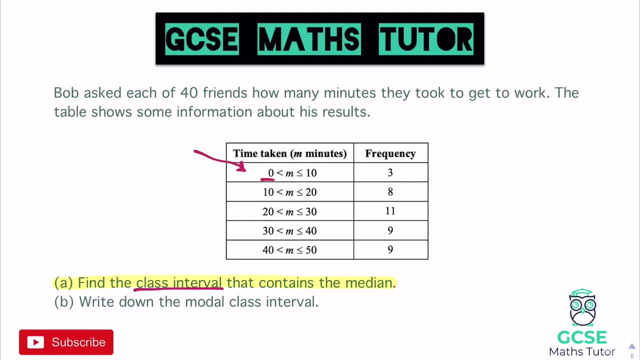 is just the language for the for being between 0 and 10.. So the interval for that is between 0 and 10, so the class interval is the group between two numbers. So basically, if we turn that into sort of simpler words, So we're looking at the class interval. 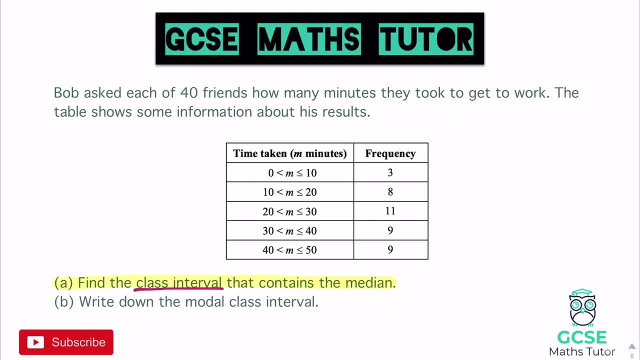 that contains the median. Now the median, hopefully you already know, is the middle number. So what we're gonna have a look at actually is how we get the middle number from a table. Now it says up here that there's 40 friends. 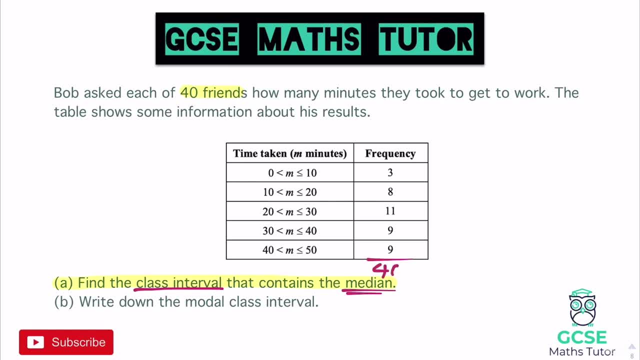 Again. if it didn't, we know how to find that. now We can go down to the bottom and find that there's 40. Now, when we're finding the median of anything, the statistical way of doing that is we add one and half it. 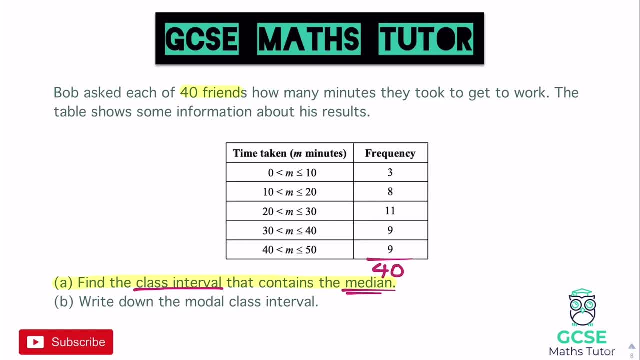 If you think about a little bit of a logic here, if we have five people, let's just draw a little picture here. If we have five people standing in a row, oh dear, I've committed to drawing five people now. All right, here we go. 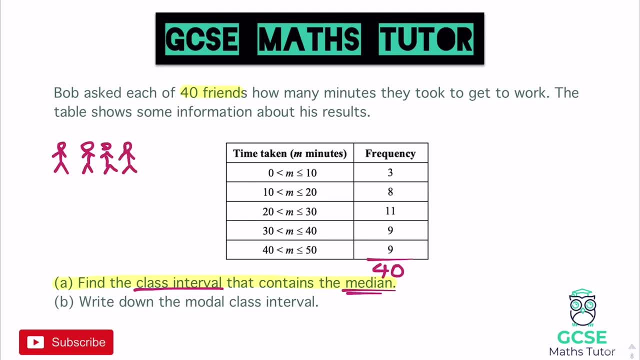 Draw them as best as I can. Okay, five amazing little drawings there, And we wanna find where the middle person is. Obviously, logically, we know that that middle person is this one right here, the third one along, But if you take five people and divide that by two, 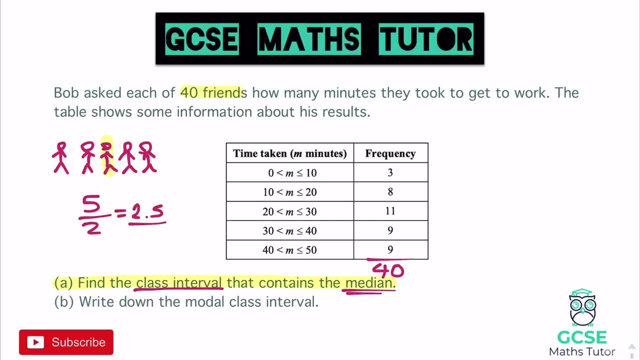 you don't get three, you get 2.5.. So it doesn't actually find that middle person. So actually the logic we have to take is: before we have it okay, we have to add one, So five plus one, which is six. 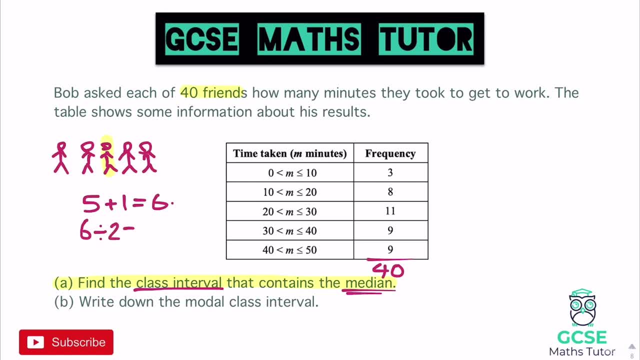 Then we divide it by two. Six divided by two tells us that the middle person is the third, and that is correct. Look, one, two, three, our middle person, four, five. So when we're finding the median, hopefully that is a nice little simple example. 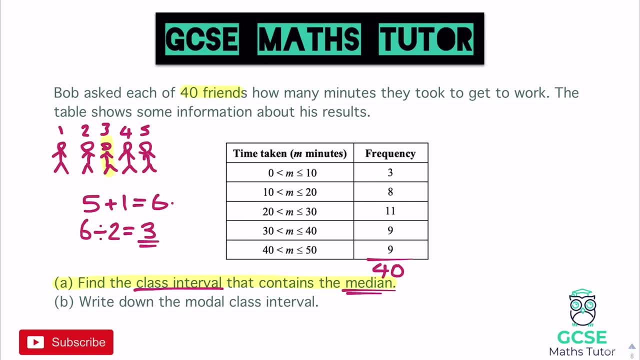 as to why you add one, but we have to add one first and then actually have it to find out where our middle value is gonna lie. So let's have a look Now we've got 40 people, So 40 plus one is 41.. 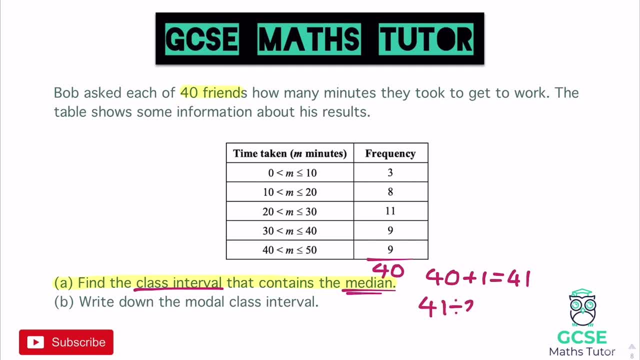 And then we're gonna half that. So 41 divided by two is 20.5.. So we're gonna try and find where the 20.5th number is, and that seems a little bit weird. Sometimes it's a bit easier just to half 40,. 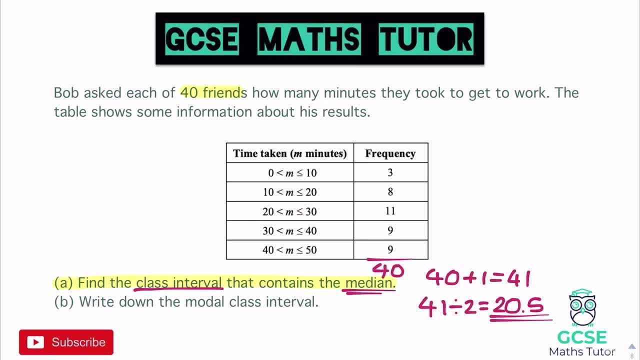 but mathematically that's not actually correct and it's not gonna be a good way to learn this as it progresses onto other topics, when we start to look at things like box plots and stuff like that and stem and leaf diagrams and all that sort of stuff. 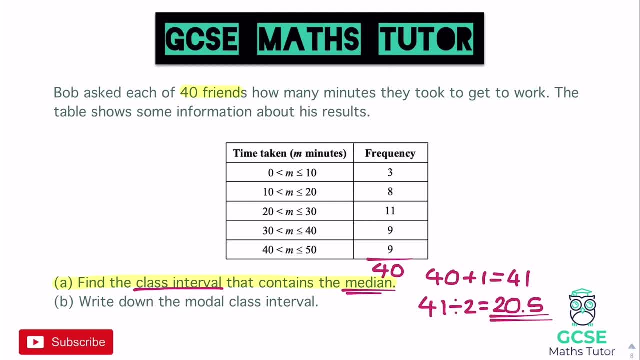 So let's have a look. The 20.5th number. Now what we're gonna do is we're gonna do something called a cumulative frequency here. So what I mean by that is we're gonna do a running total down the table. 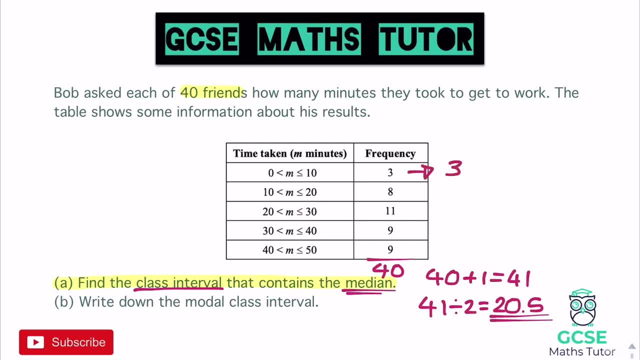 So as it stands on this first column, look, we've got a total of three Once we add in this extra eight here. well, three plus eight gives us 11 people in total now. so we've not quite got to that 20.5th person. 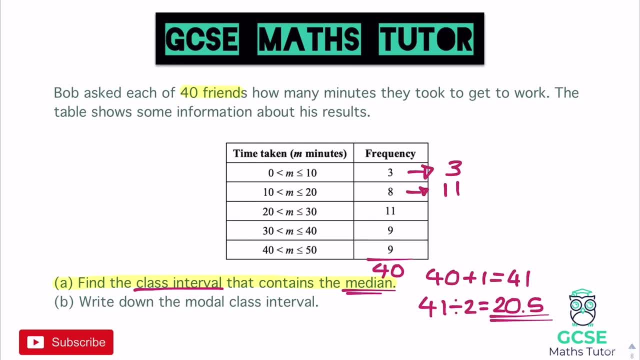 Not that we can have half a person, but just in terms of our median. we've not got to that 20.5th number yet. Once we add the 11 in, that gets us, say it gets us to 22,, and that has just gone. 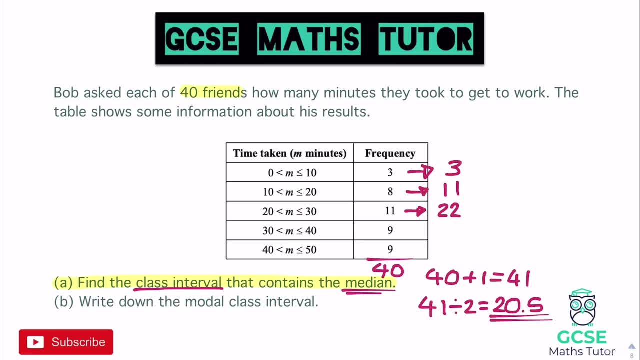 beyond the 20.5th number. So there we go. that 20.5th person is somewhere within that little category there. Okay, obviously not in the category above, because we're only at 11 people by then, but as we progress down the list, 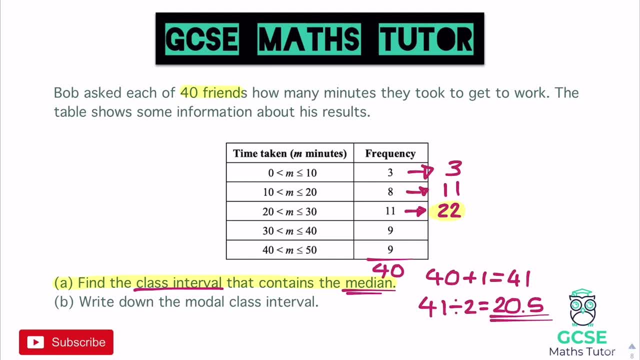 that 20.5th sort of person there is gonna be in that third category. So that leaves us with a median in this category here. So our median class interval is gonna be that 20 to 30 right there, And when we write down, 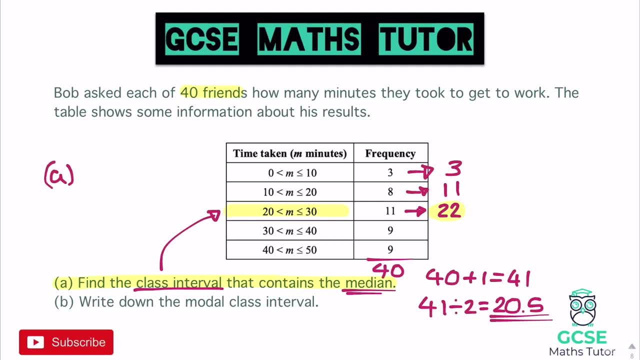 our answer for that. so for part A, we would literally just write down exactly what is written right there. So 20 with our inequality to 30, and there we go. there's our median class interval. okay, So what we do is we get our total, add one half of it. 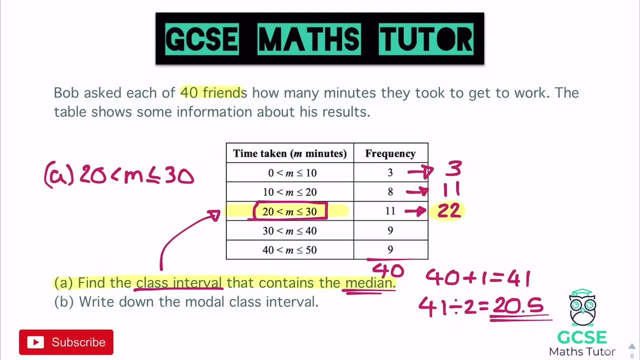 and then we count down our list using cumulative frequency to figure out where that person actually is, And we just wait till we've gone just beyond it. and that's the category that they're in The next part here the modal class interval. 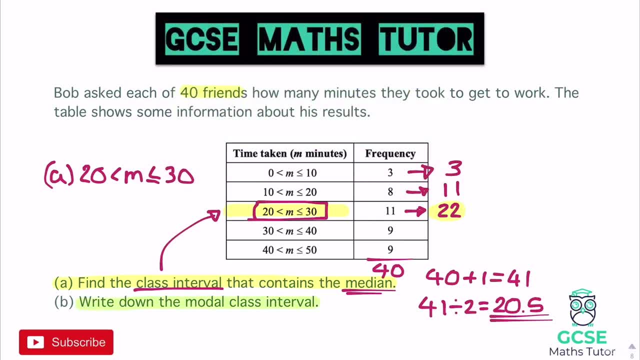 is a lot easier. Write down the modal class interval. Now that word modal just stands for the mode. there we go. but because it's referring to a class interval- again just one of these groups- we use the word modal. okay. 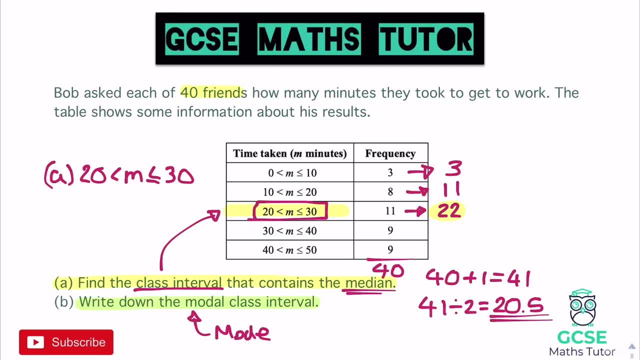 So write down the modal class interval. Now, that's nice and easy to find. All we have to do is look down our frequency and see which one is the most popular. okay, The mode is the most frequent. okay, If we write that down most frequent. 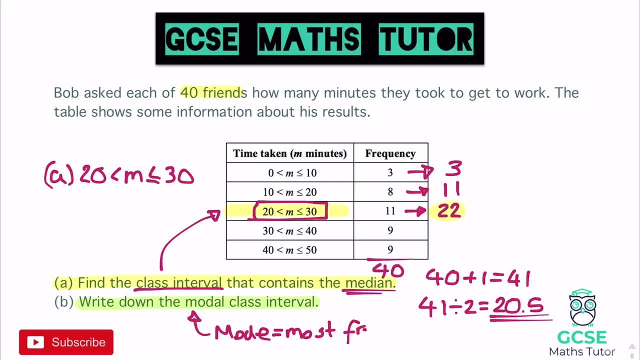 or the one that's the most popular. okay, I tend to use that word popular rather than frequent, but that is the mathematical language there, the most frequent, And if we look down our table, we've got three, eight, 11,, nine and nine. 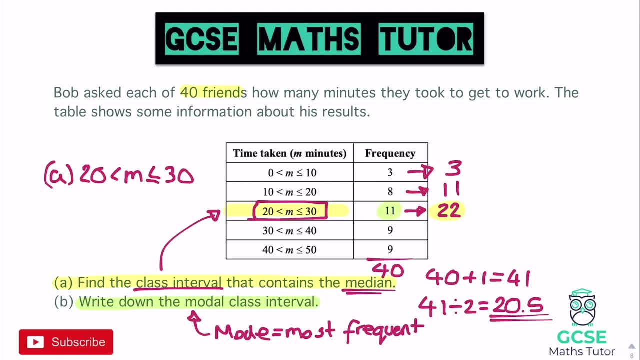 11. there is the most frequent, okay, the most common. So our modal class interval is also that particular category there, which ends up being the same as our median in this particular question. So our part B: there we'd write down the same thing. 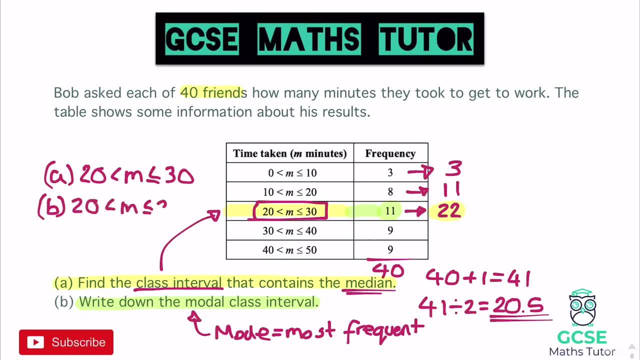 We'd say 20 to 30, and that is our modal class interval, our most frequent. okay, And this same logic applies when it's a non-grouped frequency table. Obviously, when it's non-grouped frequency it won't say: write down the modal class interval. 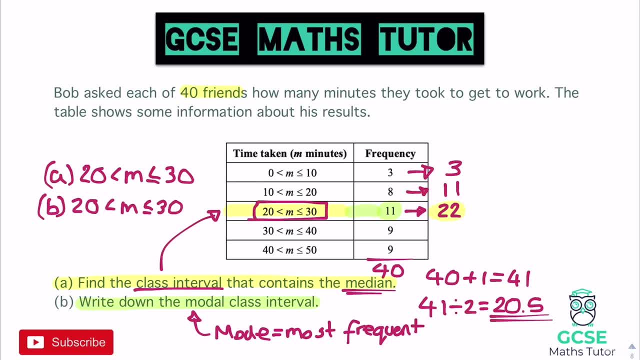 or the median class interval. It would just say: write down the median or write down the mode. okay, Okay, but obviously it's a little bit trickier when you've got to write down the actual interval, but the process is exactly the same. 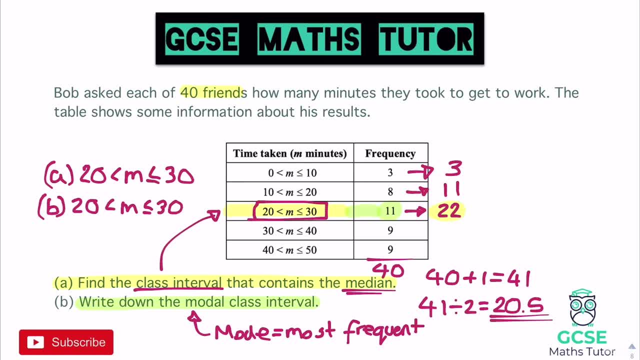 on the other table as well. So we're only gonna practise on these particular tables because they're a little bit trickier just in terms of what you have to write down. But, honestly, both the questions are exactly the same here, but I've just chosen to actually go with these ones. 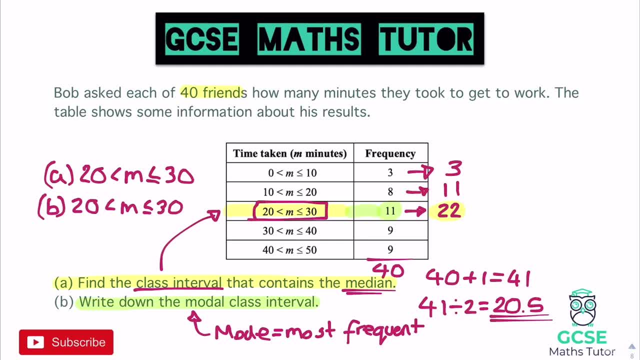 as they're a little bit more popular when you're asking to look for the median or look for the mode, Okay, so that is how you actually go about doing that. In terms of the actual range, the range is quite nice and easy. 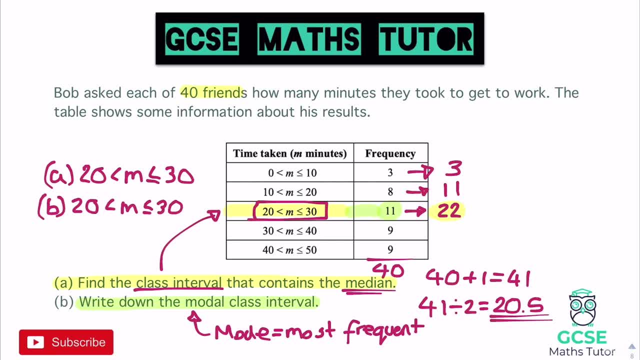 I'm not gonna actually get you to have a go at these because they're so nice and simple. Obviously, when you're looking at the range, you just do the biggest, take away the smallest. and our biggest time, take away our smallest time. 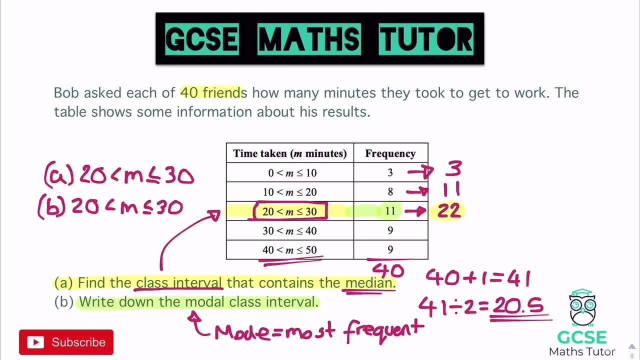 Obviously, if there were numbers in here then we could just do the biggest one down here, take away the smallest one up here. But as they are classes or groups we can't do that. so we estimate the range. We would do the midpoint, the 45 midpoint. 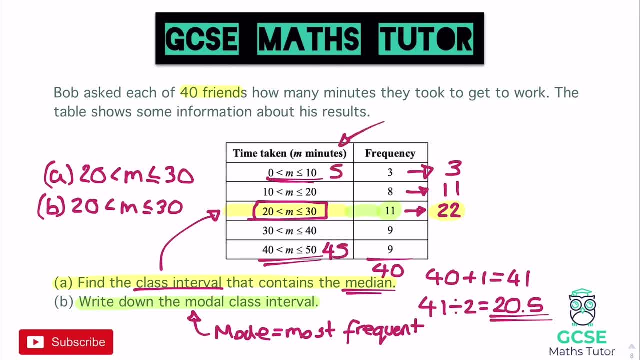 take away the five midpoint up here, So to estimate the range. it's an estimated range. here We'd do 45, take away five and our range would be 40. Really nice and simple to work out the range. but we're gonna focus on median and mode. 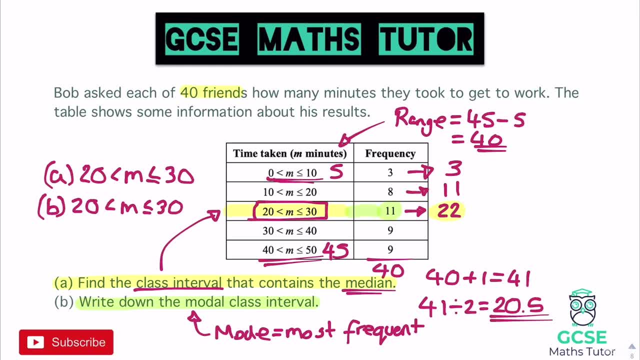 But that is how you work out all the averages from one of these tables, Okay, so what you're gonna do is you're gonna have a practice on working out the median and a practice on working out the mode, okay, and figuring out those. 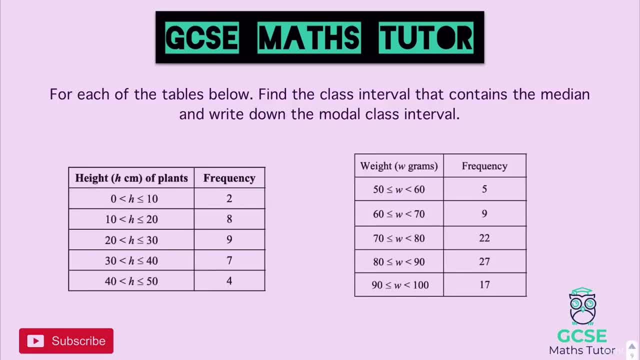 So here they are. Okay, so there's two questions here Now. hopefully you've been writing these down and, if you have, you've already got these tables actually written down somewhere, because these are the last two that you just looked at. 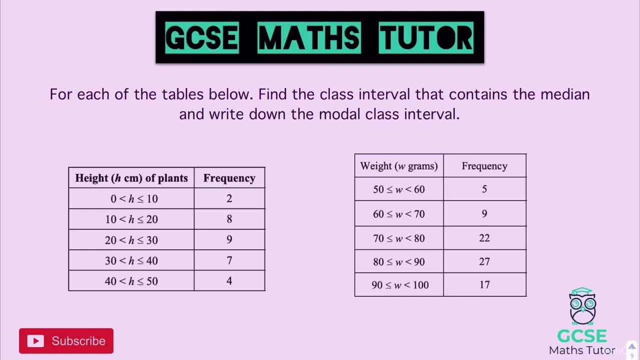 So those last two tables that hopefully you've written down, I want you to have a look, I want you to find the class interval that contains the median for both of them, and also I want you to write down the modal class interval for both these tables. 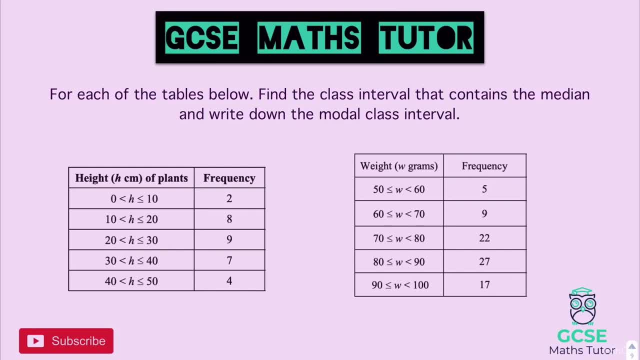 So pause the video there, have a go, and we'll go over the answer in a sec. Okay, so starting off on this one on the left, then I'm gonna start off finding the median. So if we add these all together and see how many we've got there, 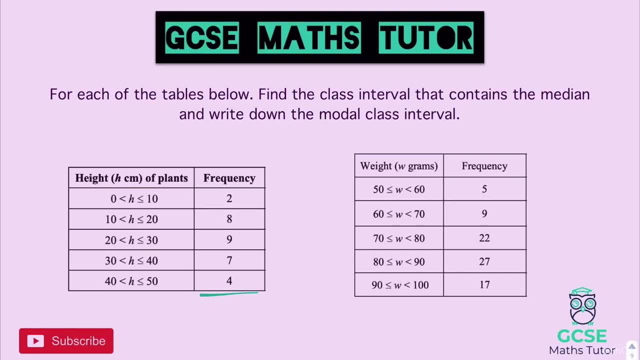 So we've got two plus eight plus nine plus seven plus four, and that adds up to a total of 30. So to find our median, we'll add one, which is 31,, and divide that by two, So we end up with 15.5,. 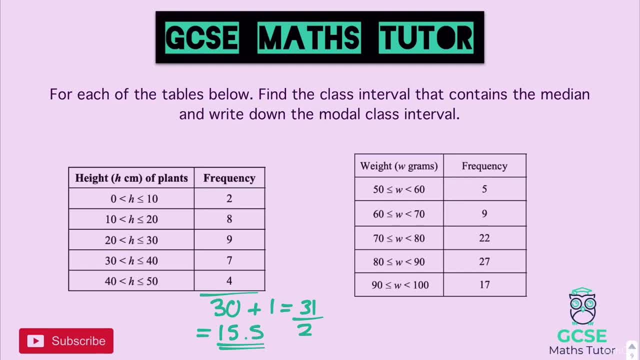 and that's where our median is gonna lie. So if we do our running total going down the table, we have two here: plus the eight, that gets us to 10, plus the nine that gets us to the 19.. 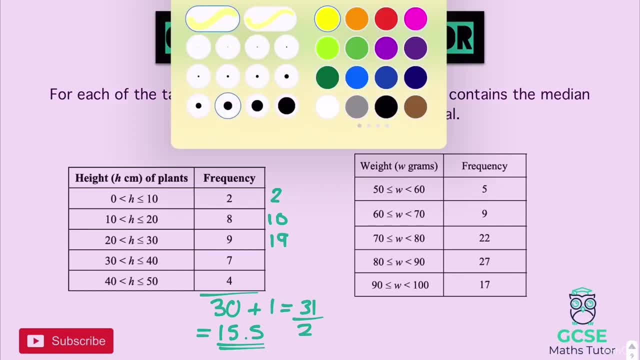 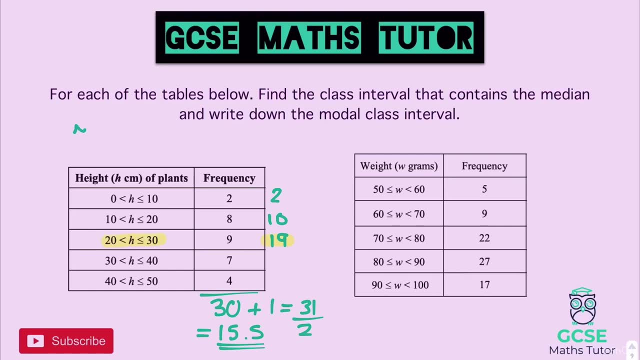 There we go. So we've gone beyond 15.. So our median is gonna be within this category and that is 20 to 30 there. So I'm just gonna write this at the top here: Let's go for our median, which is gonna be 20.. 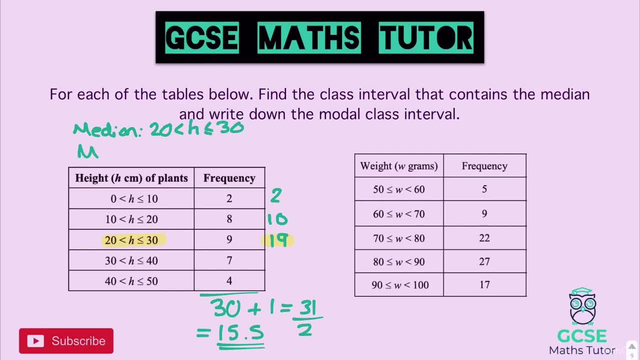 There we go to 30. And then we'll also look at our mode. Okay, obviously we are looking at the median class and the modal class, but I'm just gonna shorten that down just as I write these for you, Right? so on to our next little part, then. 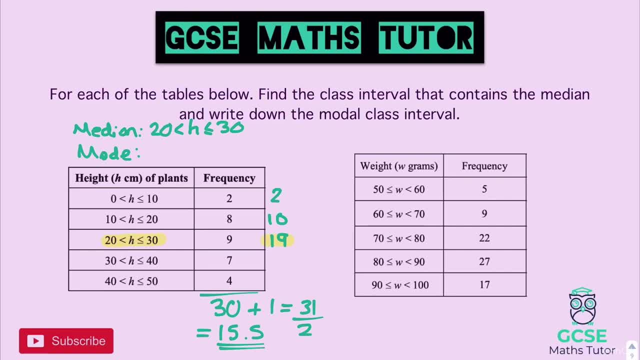 Let's have a look, let's go for a different colour. We are gonna find our modal class, and a modal class is nice and easy. We just have to look at our frequencies and see which one's most common. So 28974, nine, there is the most common. 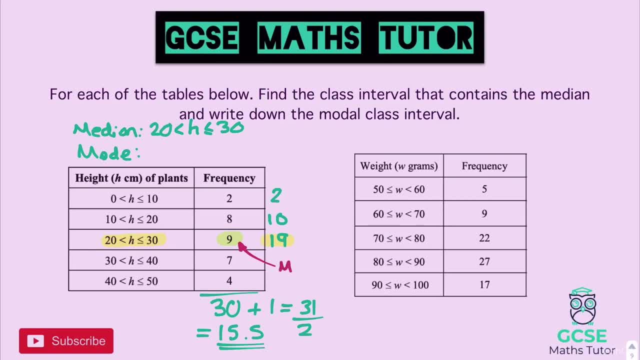 So that's gonna be our most frequent, or our modal class. There we go Now. obviously, you've just gotta be careful. Obviously, our mode isn't nine. Nine represents how many are in that category, But the actual category is on the left here. 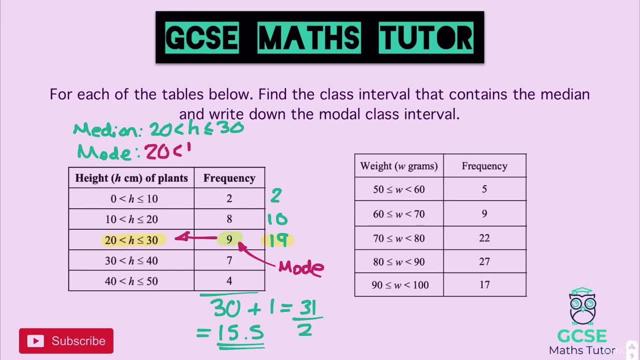 So our most common category is also that 20 to 30.. And just a little side note here: they're not always the same. It's not always that the median is also the mode. It just so happens that these are obviously are ending up being the same here. 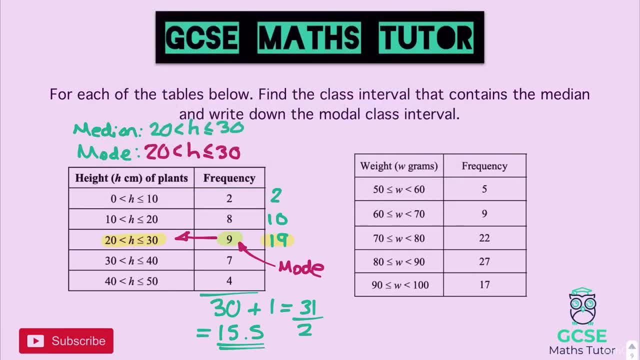 but they could be different. Onto the one on the right, Let's have a look. So let's get our total. We've got obviously larger numbers in this one. We've got five plus nine plus 22 plus 27 plus 17.. 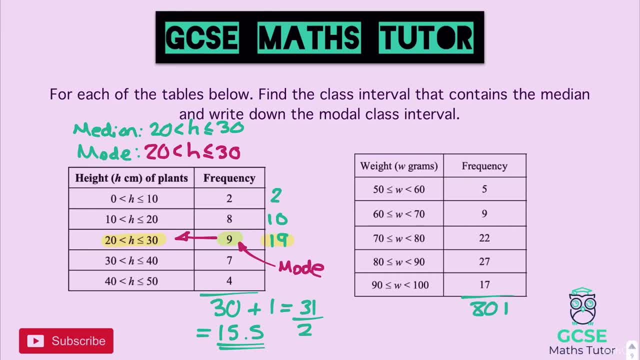 And that gives us a total of 80. So if we add one it gives us 81, and half of that is 40.5.. There we go, So that's where our median's gonna be. So counting down the list there. 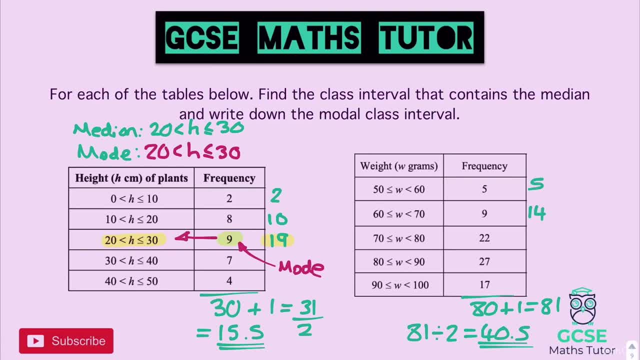 we've got five plus nine, which is 14,, plus the 22,, which gets us to 36.. Still not got to our 40.5.. But once we add the 27,, 36 plus 27 is 63.. 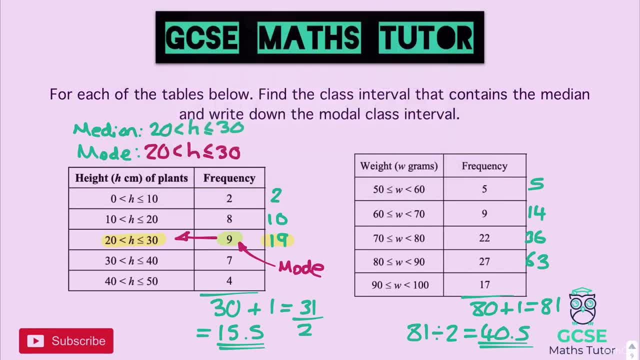 So we've gone beyond the 40.5 there. So that is where our median's gonna lie, and that is the 80 to 90 category. So our median, our median class, is 80 to 90.. There we go. 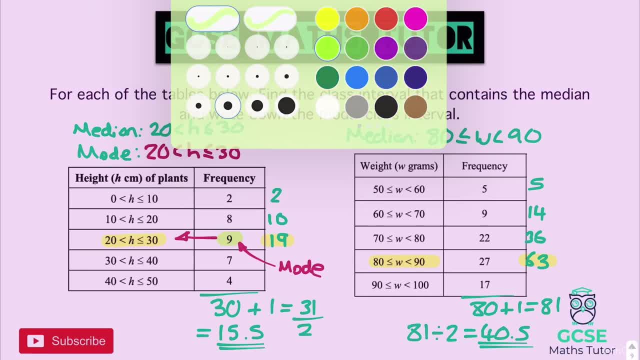 And that's our median. Now, looking at our mode, let's have a look which one's our most common. We've got five, nine, 22,, 27, and 17.. And there we go As it turns out. look, the mode is also. 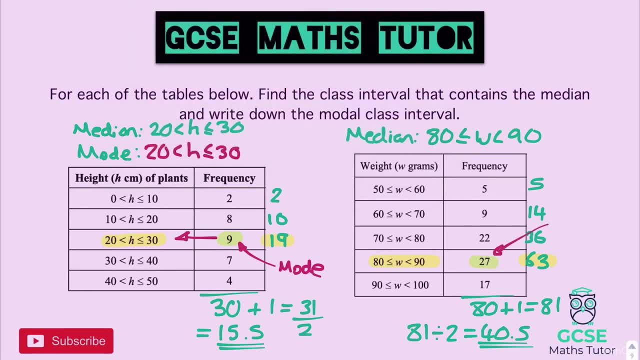 in exactly the same place. There we go. So that's our mode, or our most frequent. So our mode or class is this one on the left, just here. So I'm not gonna write that down again. I don't think there's actually anywhere I can fit this. 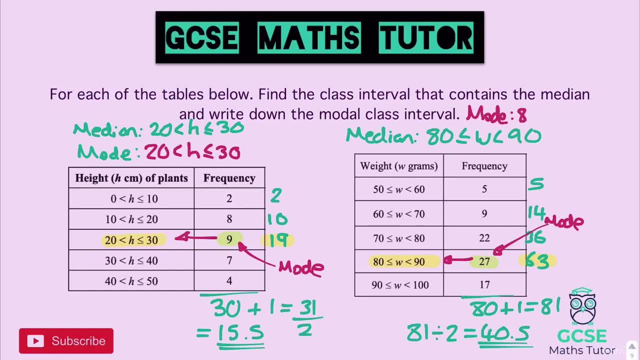 Let's just write it up here. So our mode, there we go. We would just write 80 to 90. Obviously using our inequality there. that's shown in the table, And there we go. That is our mode for that second question. 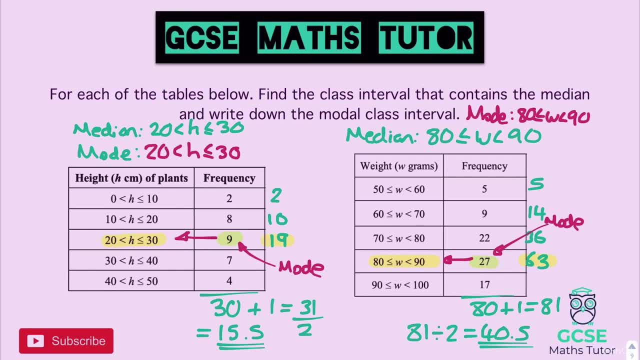 And there we go. That is how you find all the averages from a table. Obviously, you could also look at the range And just to finish this off very quickly, our range for this first table: look, we could have five in the middle and 45 there. 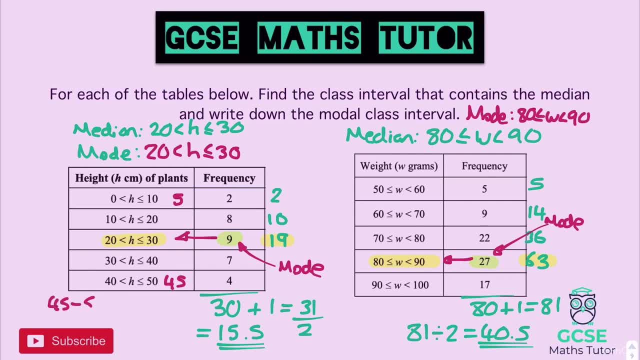 So our range would be 45,. take five and our estimated range- sorry, there would be 40. And our estimated range for this one on the right: look, we would have 95 in the middle of that one, 55 in the middle of that one. 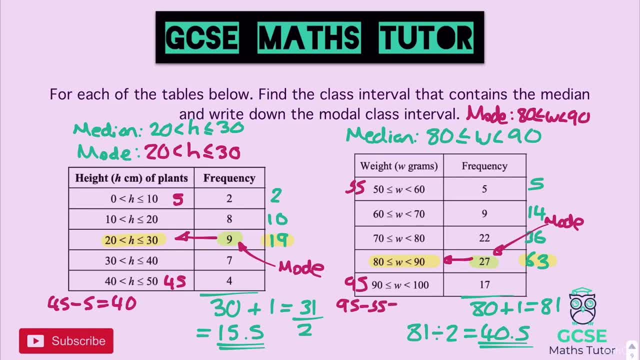 and 95, take 55, would give us an estimated range of 40.. There we go, And there would be our estimated ranges. There we go, And they turned out to be the same number for both questions. But there we go. 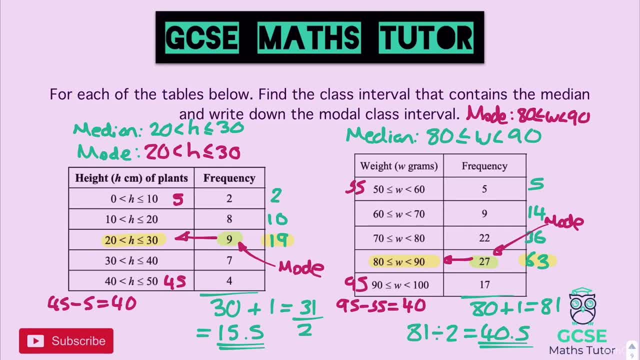 That is finishing all of that off. That is all. the averages We looked at mean from a normal frequency table, mean from a group frequency table, and then obviously looking at the median and the mode and the range from these grouped frequency tables. And again, don't forget that, if you do have